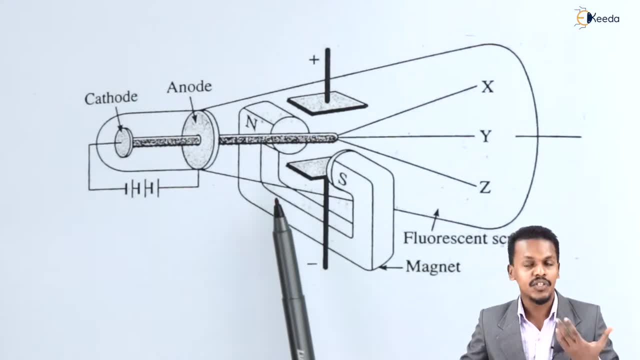 induction and this is nothing but the magnet which will produce that is magnetic field. Suppose if the external forces, that is, the electric field and the magnetic field, the both are not present and in the absence of that, obviously the cathode rays. we understand about the property of it, that is, it travels in a straight path from cathode to anode, So that 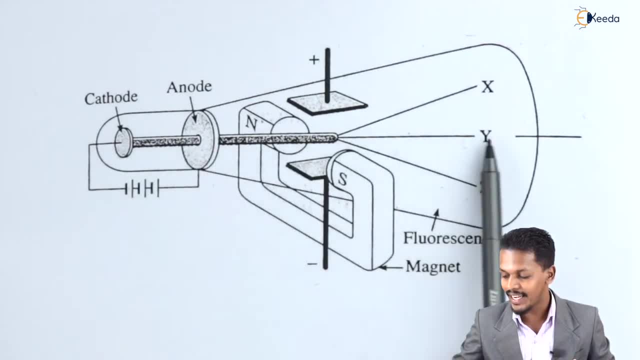 is how basically the cathode it will be passed in a straight direction and it will hit the tube and that is how basically this tube is made up of. that is ZNS screen and that's the reason this part, that is the point why it will try to glue. So this happens when the cathode rays travel in absence of 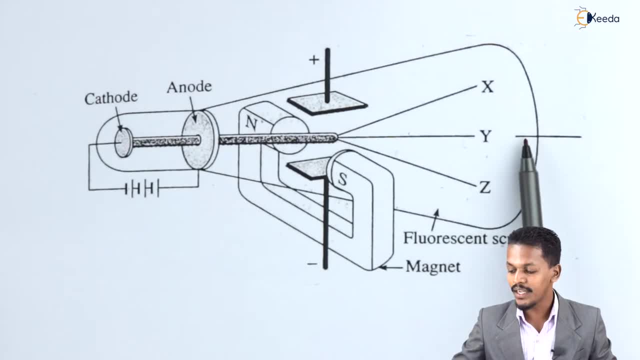 external field and that is how, basically here, that is at point Y, will get the glue. But what happens if we turn on the electric field and will switch off the magnetic field? so in that case, basically we understand, that is the cathode, that is the cathode rays are nothing but the. 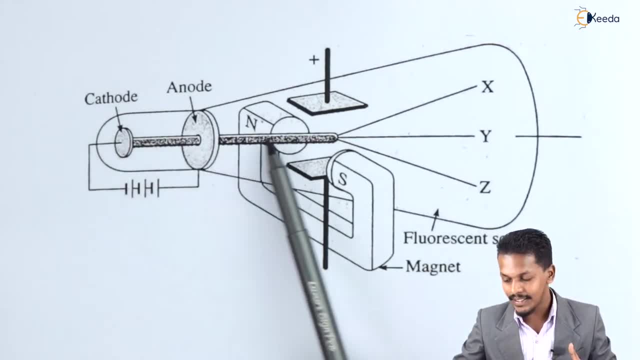 electrons and obviously, whenever they will pass through this tube, whenever the electrons will come over here, obviously they will, that is, they will try to attack with the positive charge plate and that is how, basically, the cathode rays, in spite of traveling in a straight direction, they will deviate. 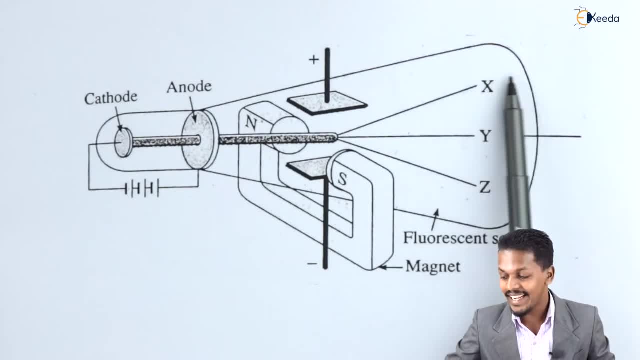 a bit and it will hit the point X and this point X, it will glow. So this also shows the factors that are depending on the deviation of the cathode rays. So this is one of the point that is what we have discussed, that is, the electrical field. So this is how, basically, we'll get a glow at point X. 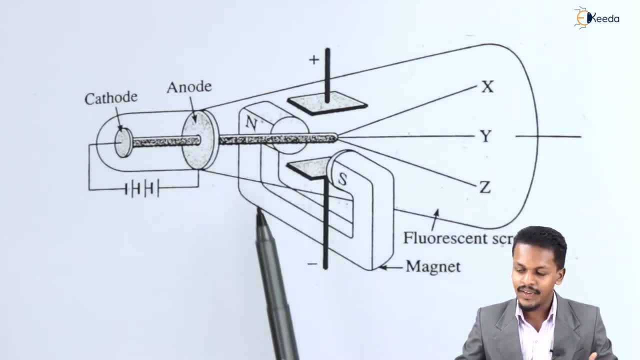 Suppose, in the another study, we turn off this electric field and we turn on this magnetic field. so in that case, whenever the cathode ray is basically passed through this tube, we could find that is the cathode ray, that is, the electrons. it will deviate and it will hit. 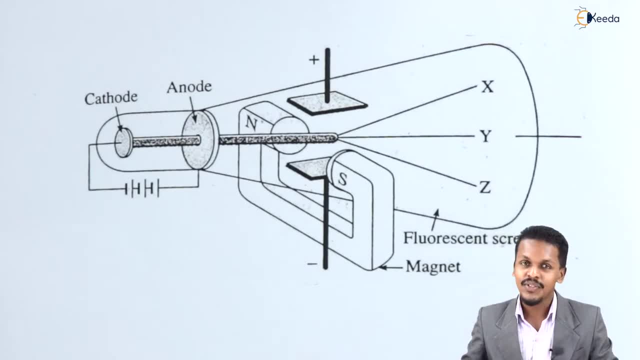 the point Z and here, basically, there will be a glow. so therefore we could get three glows at three different experiments or three different study. that is, in absence of the electric and magnetic field, we could find the glow on the y point. in presence of the electric field, we could.